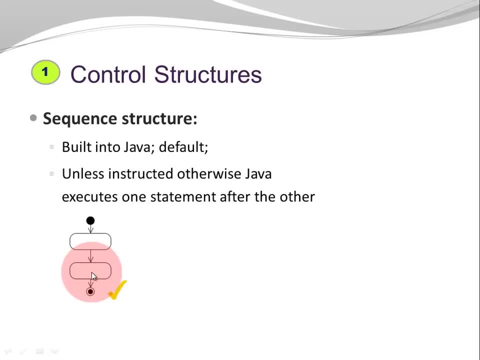 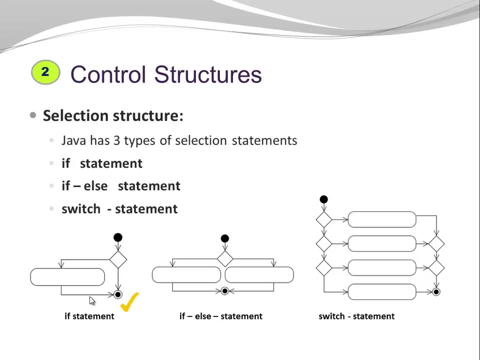 We execute one action after the other or one instruction after the other, Until we reach the end, which is the final state here. The second control structure is the selection structure. Here we choose a certain path of execution based on a condition. 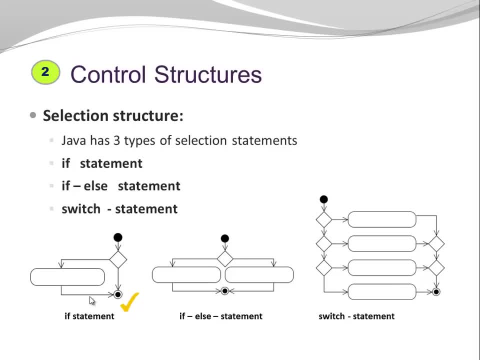 Java has three types of selection statements: The if statement, the if else statement and the switch statement. Each of these statements has a corresponding activity diagram. Let's look at the if statement. I start. I reach a decision based on my condition. 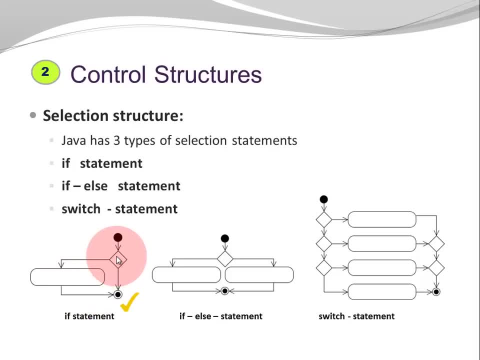 I execute some code- or maybe not- In my if statement. I execute some code In my if else statement. I start, I reach a decision Based on my condition. I do one thing or another and then I'm finished. 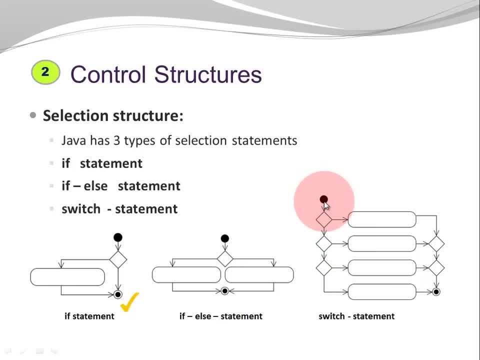 Here in my switch statement I start. I reach decisions to be made. In a switch statement, I compare a variable to different values and depending on the value of my variable, a certain path of execution is chosen. So here I have a number of different choices and then at the end they merge. 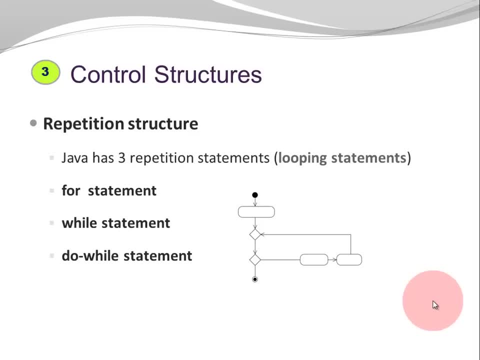 This is it. The third control structure I want to talk about is the repetition structure. The repetition structure allows me to repeat a code segment over and over again. In Java, we have three repetition statements: The for statement, while statement and do while statement. 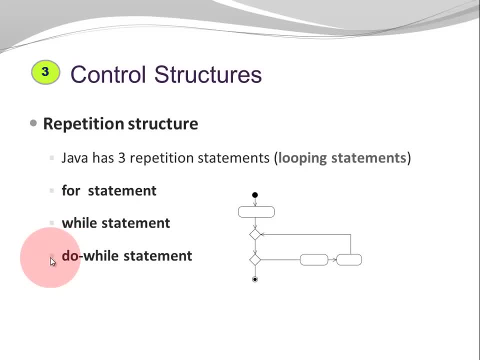 They are also referred to as looping statements or just loops. By the way, there are two types of for statements or for loops in Java, but at this point I don't want to go into that. I do want to show you a corresponding activity diagram, though, so this activity diagram here can 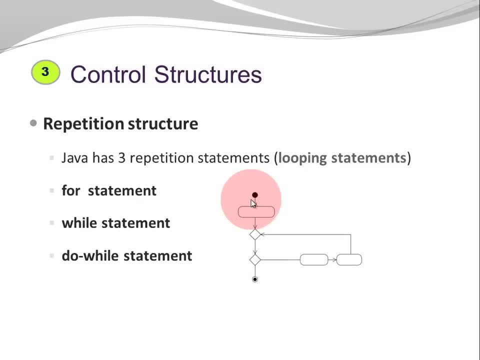 represent a for statement. This is a for statement. This is a for statement. This is a or or or a while statement. We start, We initialize the control variable and we keep repeating as long as my condition here is true, and then, when this condition is no longer true, and move. 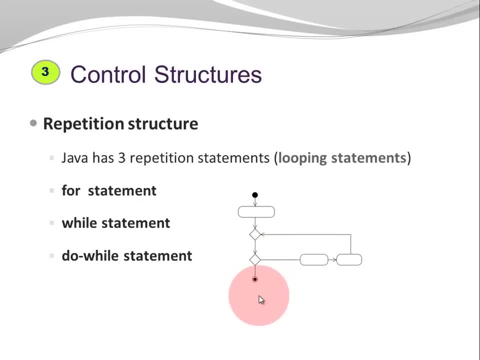 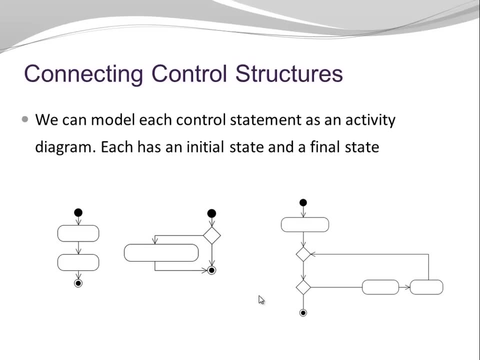 on to the final state, to the end. At this point we looked at different conditions and control statements corresponding to the three control structures. all of those are still fairly simple. However, they can be combined to represent more complex scenarios. We saw that each of the control statements can be modeled. 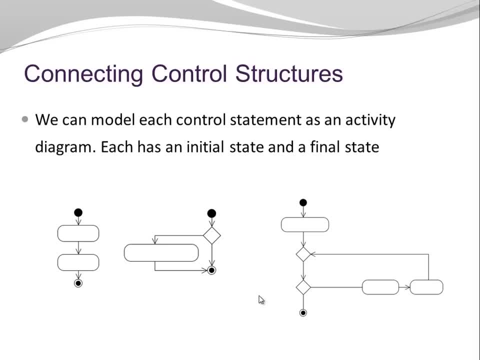 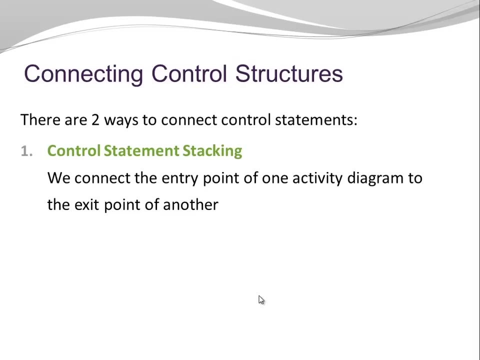 with an activity diagram, and each of those activity diagrams has an initial state and a final state. We can combine and connect control structures in two ways: by stacking and by nesting. So first let's look at control statement. stacking- It is easiest to visualize, when you think. 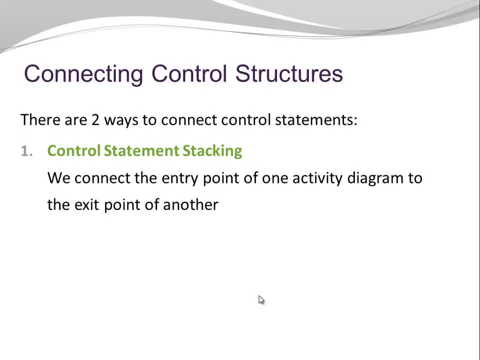 of your control statement in form of the activity diagram representing it, So we can connect the end of the entry point of one activity diagram to the exit point of another. Let's look at an example. Here I have a sequence statement and a selection statement. 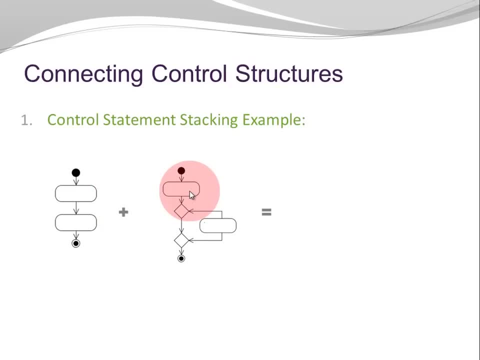 And I would like to combine those two by stacking them. Notice how I connected the entry point of my selection statement to the exit point of my sequence statement. So here you can see the sequence statement in blue, the selection statement in red, and there is an overlapping area. 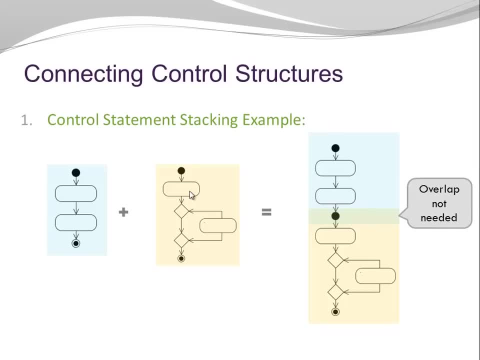 where the entry point and the exit point overlap. This overlap is not needed in the diagram, so we're going to remove it, And the solution of my stacking looks like this: The second way to do this is to connect the entry point to the exit point. 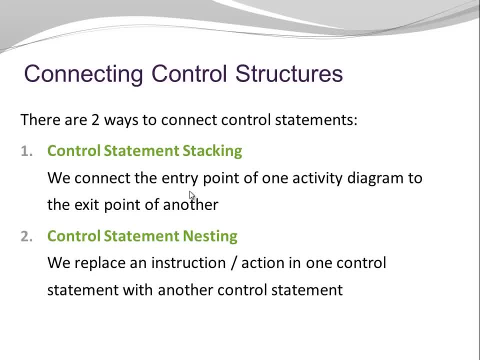 The second way to combine and connect control structures is by nesting them, So we can replace an instruction of a control statement with another control statement, or you can think of it replacing an action of an activity diagram with another activity diagram. Once again, let's have a look at an example. 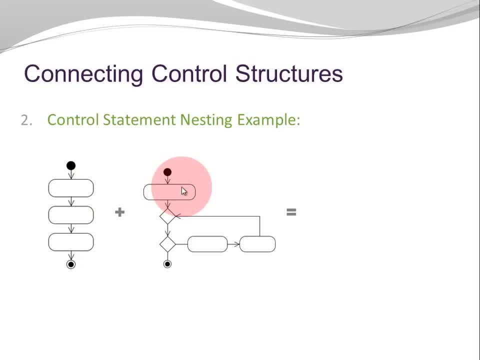 Here I have a sequence statement and a repetition statement. What I would like to do is to combine the action of an activity diagram with another activity diagram. What I would like to do is to replace the central action in my sequence statement with the whole activity diagram representing my repetition statement. 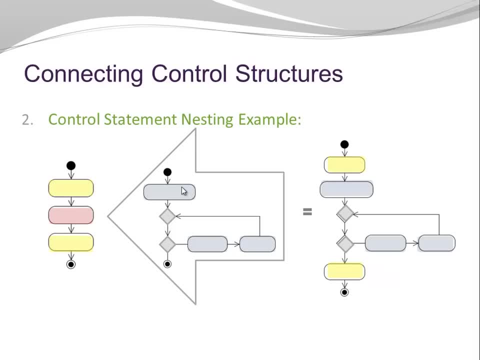 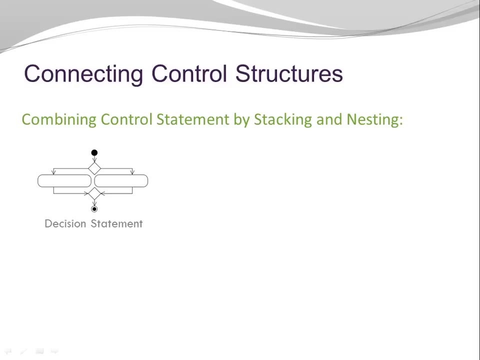 So here you can see the central action. the red colored action was removed. It was replaced by the whole activity diagram representing my repetition statement. So the last thing I want to show you is how you can use both stacking and nesting to combine control statements. 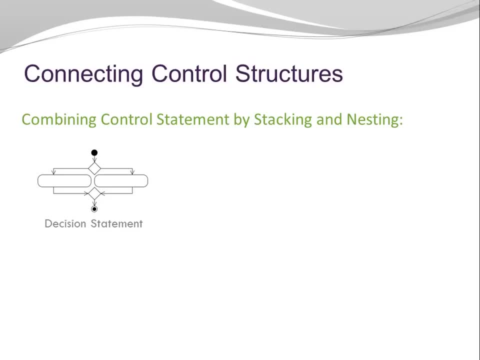 I'm starting out with a decision statement. In my case, this is an if-else statement- and I want to combine it with a repetition statement- my loop- and with a sequence statement. The way I would like to do that is by nesting them. 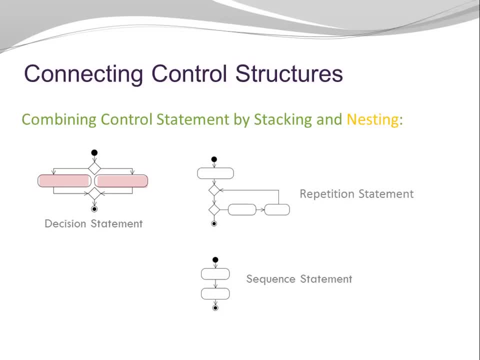 In my if-else statement you can see two actions. I colored them in red and I would like to substitute them. The left branch was a sequence statement. The right branch was a repetition statement. If I do that, I get a result that looks like the activity diagram on the bottom right. 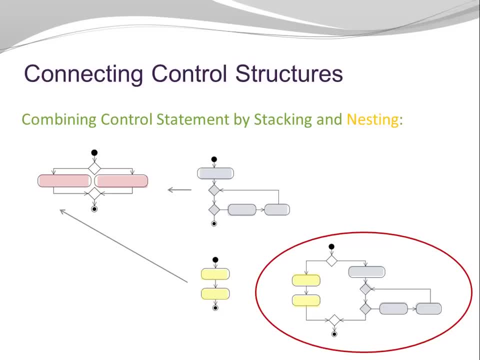 You can see the red actions have been substituted, so they are removed. Instead, I see a sequence statement. I can see a sequence in my left branch and I can see a repetition in my right branch of my if-else statement. Now I want to take this resulting activity diagram and stack it with a sequence statement.